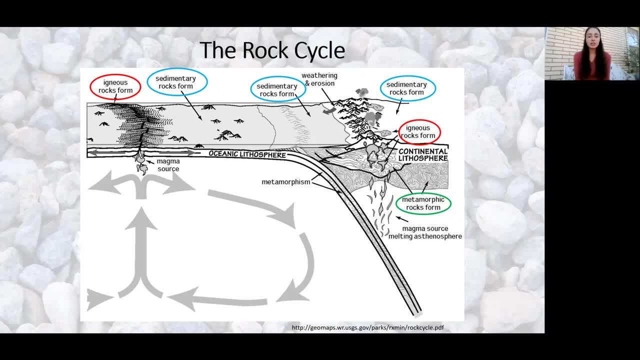 applicable to earth processes. You can see, here you've got a subducting oceanic plate and a continental plate that it is subducting under. You also have on the far left a mid-ocean ridge which will get subducted under, And then you've got a subducting oceanic plate and a continental plate. 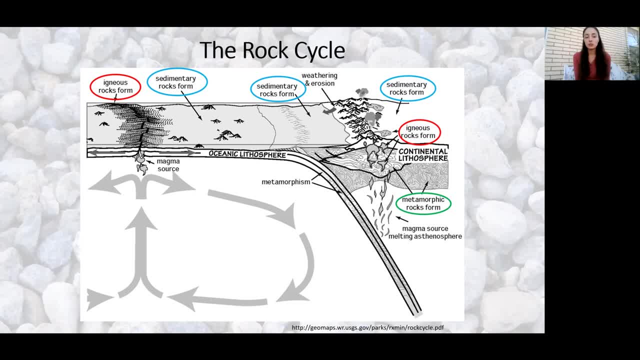 to in other episodes. Basically, it's just where new crust is forming, because oceanic plate is spreading apart and magma is coming up there forming new crust. This new crust is igneous because, like we said, igneous rocks are what form from cooling magma. Sedimentary rocks can form on. 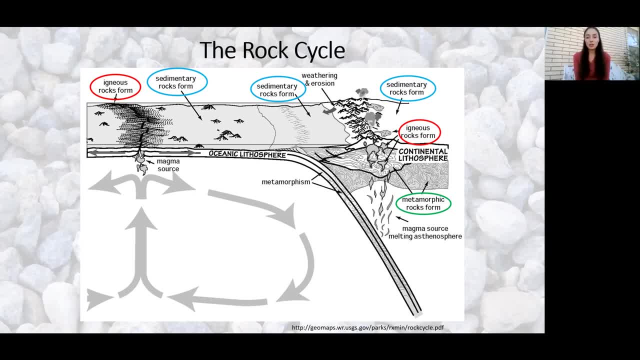 the ocean basin where sediment is accumulating and being recompacted and lithified. Lithification is just the combination of compaction and cementation. Cementation is just necessary to stick the pieces of sediment together into a new rock. You can also see that igneous rocks are forming from the volcanoes that are 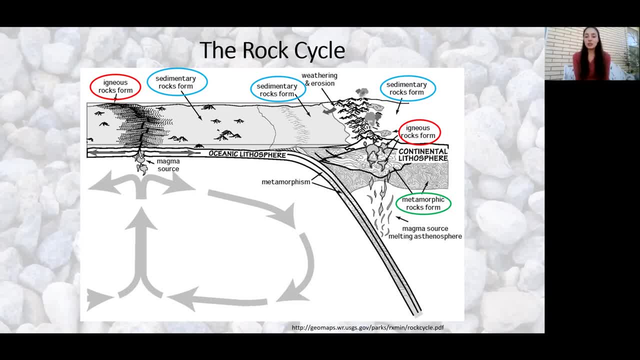 erupting along the continental edge of the subduction zone. This heat and pressure isn't only causing volcanic activity, but it is also causing deformation in the continental rocks underneath the surface. This is shown here by these squiggly lines that are metamorphic rocks. 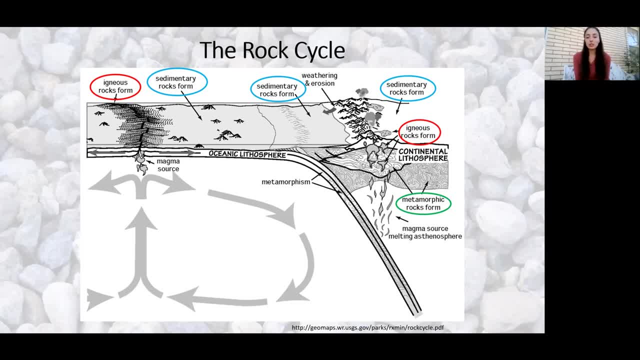 And an important distinction to make here is that metamorphic rocks only form when igneous and sedimentary rocks or even previous metamorphic rocks are put together. These rocks are put under extreme heat and pressure, but not extreme enough to melt the rock back into magma completely, because once a rock has become magma again when it cools again. 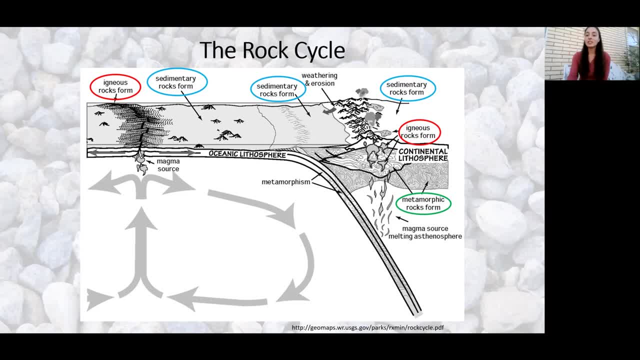 it is now deemed igneous. This also emphasizes the way that the cycle can jump around, So metamorphic rocks can be re-metamorphosed. They can even be re-melted and recooled into igneous rocks, and sedimentary rocks can become igneous again if they melt completely or metamorphic if they're. 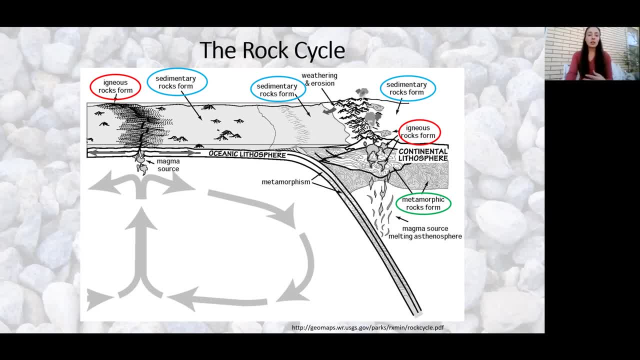 just subjected to high pressure and heat and deform or metamorphic and gaseous rock. Igneous rocks can be some sedimentary rocks from erosion and re-lithification, so it pretty much can go any which way that you see it. So now you can definitely see why these look the way they. 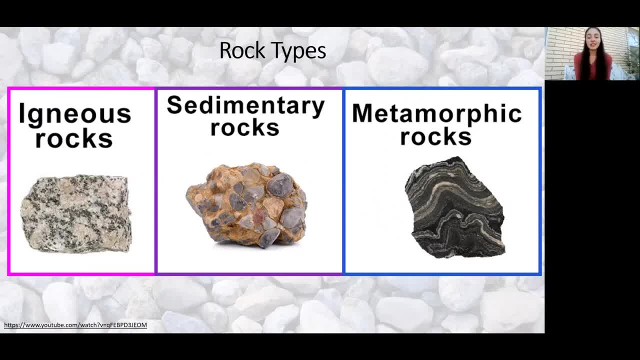 look, You can see that the igneous rocks are crystalline and the sedimentary rocks seem like broken up sediment that have been re-cemented together, like we discussed, And you can see that the metamorphic rocks look like they have all these squiggly lines, probably because they